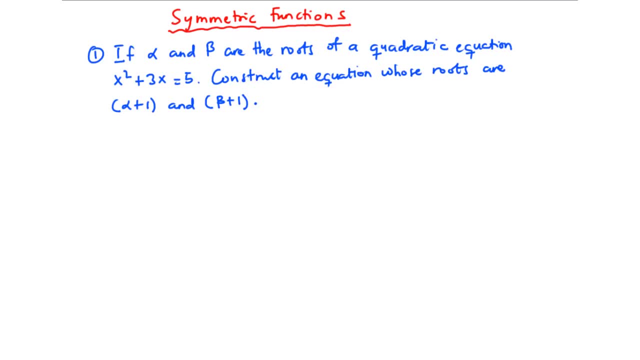 Hello and welcome back to this channel. In today's video we are going to solve some examples on symmetric functions of the roots of a quadratic equation. So in our first question, if alpha and beta are the roots of a quadratic equation, x squared plus 3x equals 5, construct an equation. 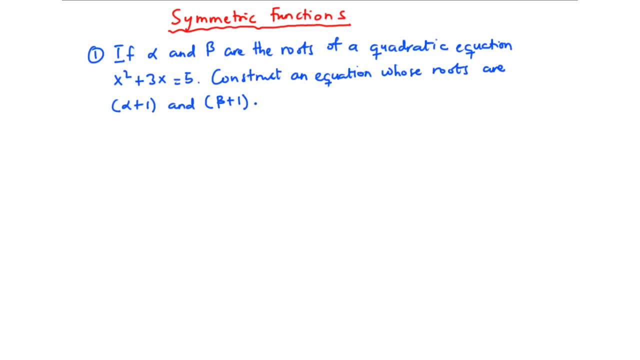 whose roots are alpha plus 1 and beta plus 1.. So this is a very simple question. however, it can look very complicated. Now we are going to solve this question. So, to solve this question, we have been given a quadratic equation with the roots alpha and beta, and then we are asked to construct: 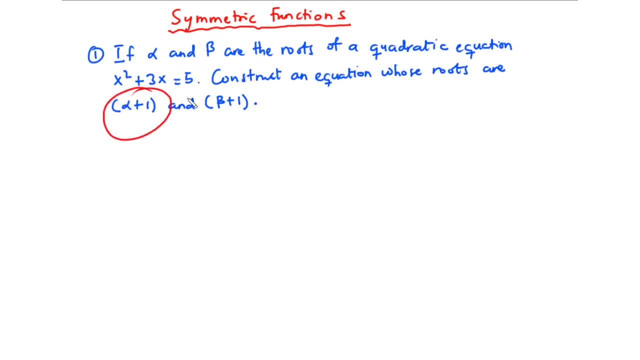 an equation whose roots are alpha plus 1 and then beta plus 1.. So we are going to solve this question with the roots alpha and beta plus 1.. So to solve the question, we are going to find the sum of roots and product of roots of this existing equation. Then, using those values, we can find the sum of. 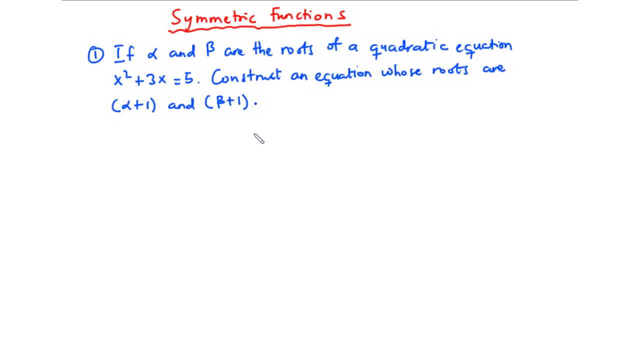 roots and product of roots of the new equation. Then, using those values, we can form a quadratic equation with the roots alpha plus 1 and then beta plus 1.. So let's do that together. Now we have the quadratic equation: x squared plus 3x equals 5.. Now we know that the general quadratic equation is given in the form. 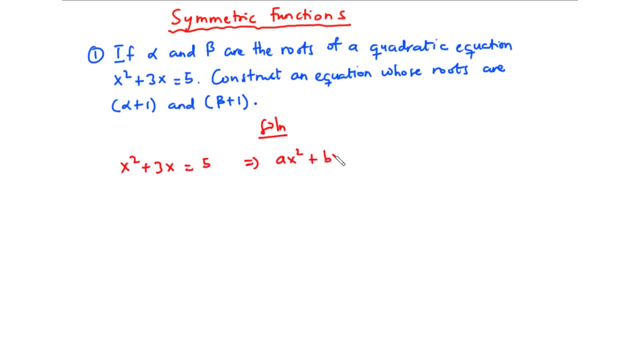 ax squared plus bx plus c. So let's represent this equation in this form. So we have x squared plus 3x, and then we need to transpose 5 to the left hand side So it becomes negative: 5 equals 0.. Now let's compare the two equations. So in that sense our a is 1,. 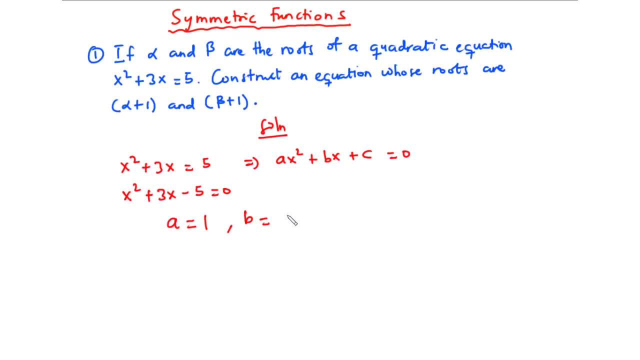 b is 3, and then c is negative 5.. So these are the values a, b and c. So let's find the sum of roots and product of roots of the new equation, of this existing quadratic equation. now we have the roots to be alpha and beta. so sum of roots. 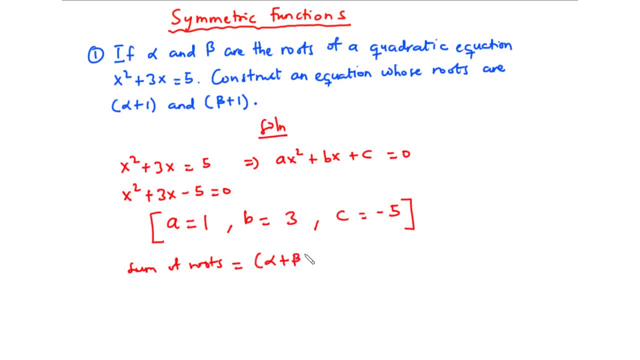 means that we have alpha plus beta, and from the previous videos we established the fact that alpha plus beta, which is the sum of roots, is equal to negative b over a. so basically we are going to substitute the values of b and a in here, so we have b to be 3, so negative 3, and then we have 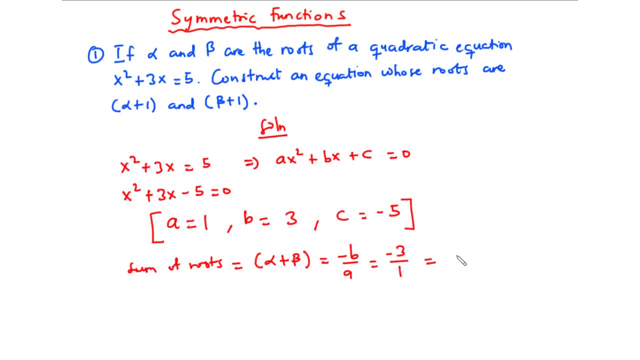 a to be 1, so the sum of roots, alpha plus beta, is equal to negative 3. now let's do same for the product of roots. so product of roots is alpha times beta, and that is equal to c over a. now we have c to be negative 5. we have a to be 1, so this is equal to negative 5. so we've been able to find the sum. 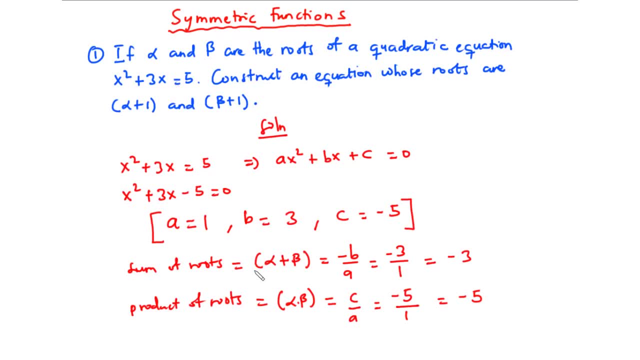 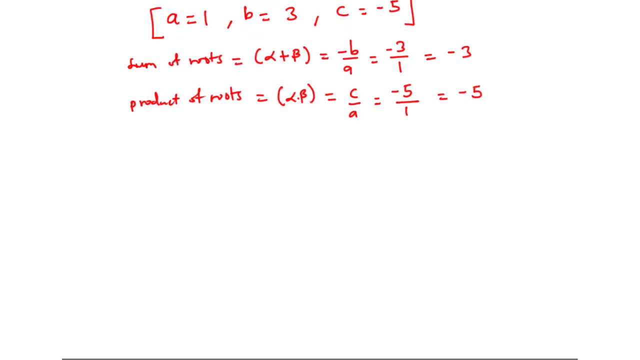 of roots and product of roots of the existing quadratic equation. now, using these same values, let's find the sum of roots and the product of roots of the new quadratic equation. we are going to add alpha plus 1 and then beta plus 1. these are the roots of the new quadratic equation we are. 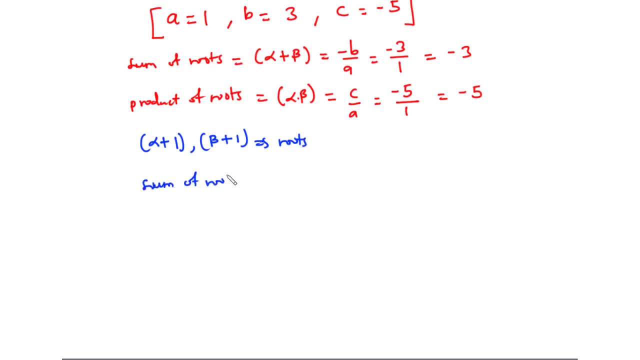 going to construct. so the sum of roots is going to be: we are going to add these two, so we have alpha plus 1 plus beta plus 1, So this becomes alpha plus beta, and then 1 plus 1 is 2.. So the sum of root is alpha plus beta plus 2.. 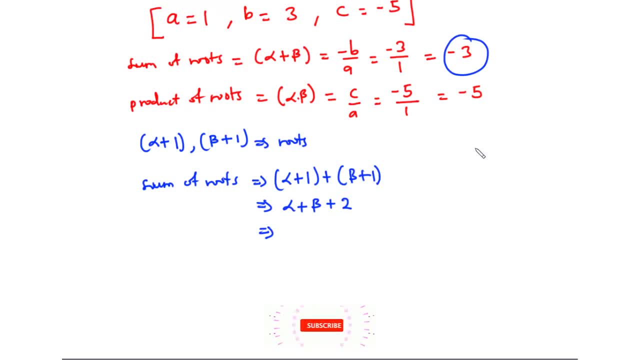 Now, from here we have alpha plus beta to be negative 3. So we are going to substitute that here. So negative 3 plus 2.. Negative 3 plus 2 is negative 1.. So the new sum of roots, The new sum of roots, is equal to negative 1.. 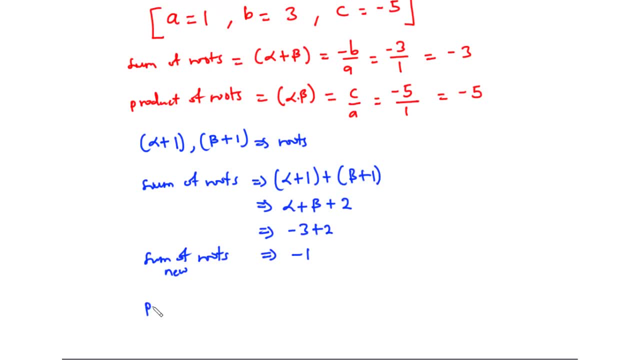 Now let's find the new product of roots. So the product of roots is equal to alpha plus 1.. Times Beta plus 1. So we have alpha times beta, alpha times 1, 1 times beta and then 1 times 1.. 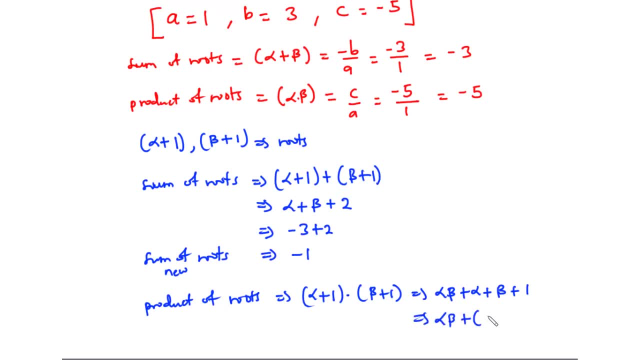 So we can simplify this as alpha, beta plus alpha plus beta plus 1. Now we have alpha beta 2. So we have alpha plus beta to be negative 5, alpha plus beta is negative, 3 plus 1. So negative 5 plus negative, 3 is negative. 8 plus 1 is negative 7.. 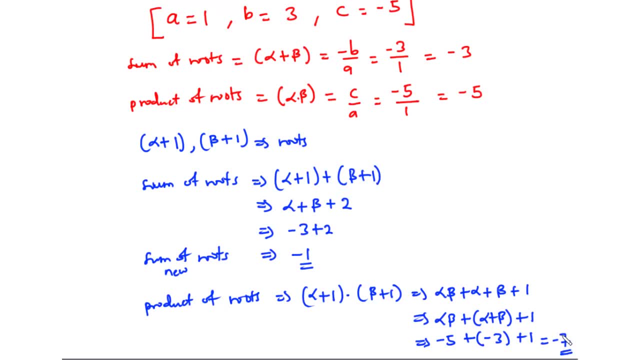 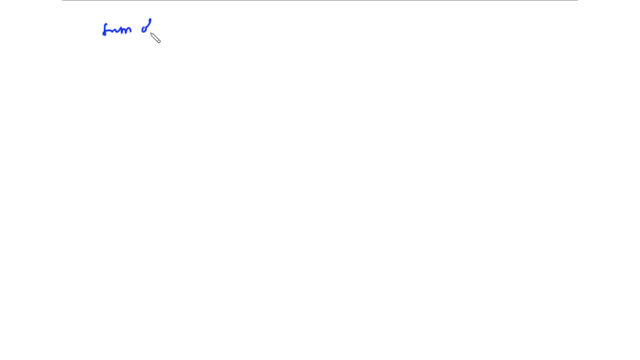 So the product of roots is negative 7.. Now let's form the new quadratic equation. So we have the new sum of roots. So we have the new sum of roots. So we have the new product of roots To be negative 1.. 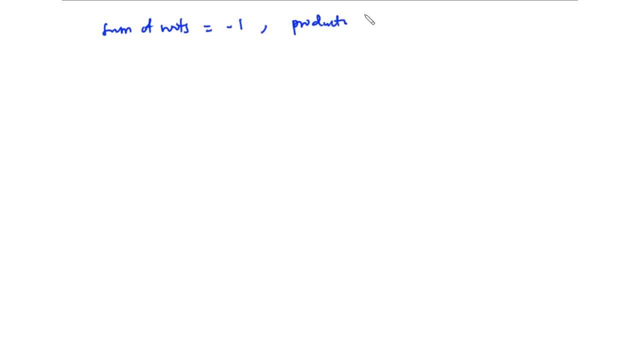 The new product of roots To be negative 7.. And then we are going to construct the new equation, The new quadratic equation. So, to construct a new quadratic equation, We are going to use the formula x square minus Sum of roots. 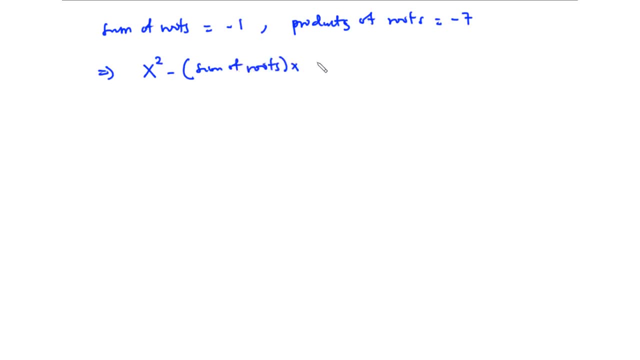 of roots times x plus product of roots equals 0.. So we have x square minus, the sum of roots is negative 1 times x plus product of roots is negative. 7 equals 0. So we have x square negative 1 times negative, 1 is plus 1.. 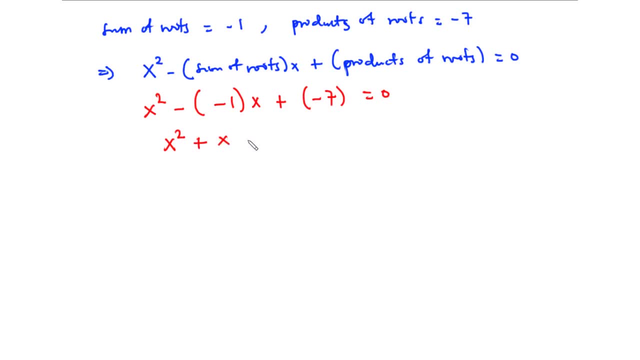 1 times x is x minus 7.. So this is the new quadratic equation which has roots alpha plus 1 and beta plus 1.. Now let's solve the second question. So for the second question, The roots of the equation- x square plus 6x plus p is equal to 0- are alpha and alpha minus 1.. 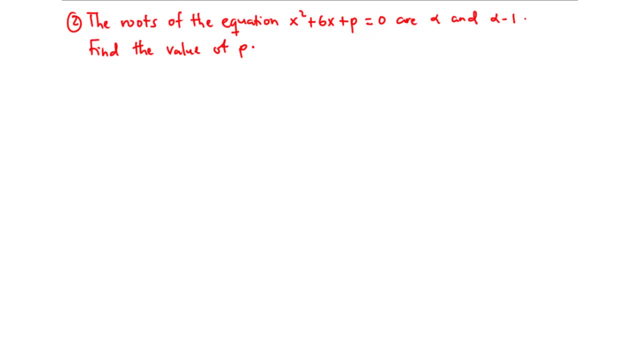 We are going to find the value of p. So to solve this question, we need to find the coefficients a, b and c of the quadratic equation. Then we can find the sum and product of roots and then, using these roots, we can generate an expression to compare and find the value of p. 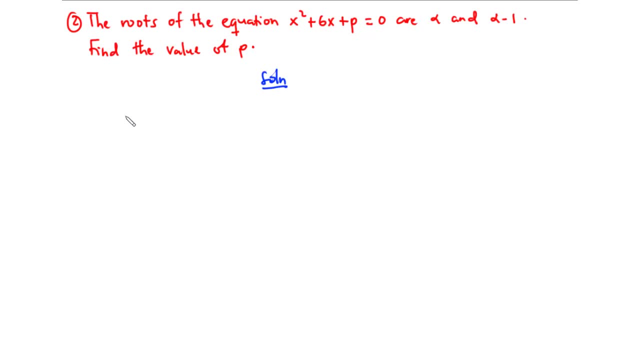 So we know that the general quadratic equation is given by ax square plus bx plus c equals 0.. And then we have the equation x square plus 6x plus p. So straight away our a is 1, b is 6 and then c is p. 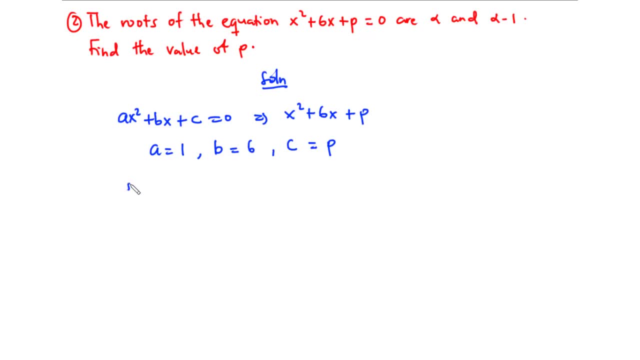 Now let's move on to find the sum of roots and product of roots. So the sum of roots is equal to negative b over a. We have b to be 6.. So negative 6a is 1.. So we have the sum of roots to be negative 6.. 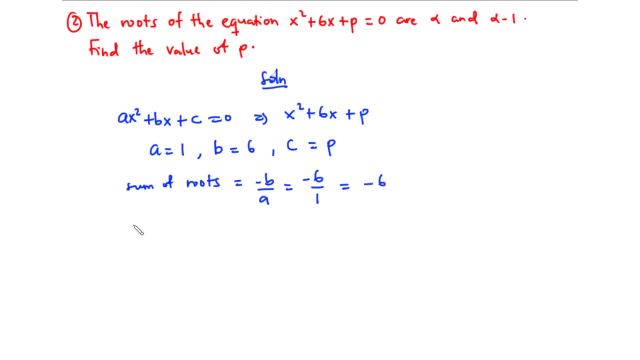 Now to the product of roots. That is equal to c over a. We have c to be p, So we have c to be 2x, So we have c to be 2x, We have c to be 2x and we have c to be 3x. 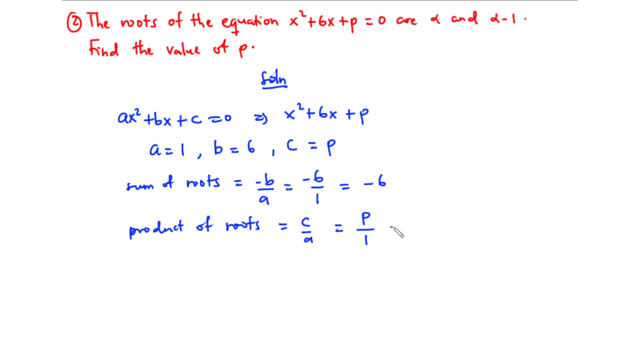 So we have c to be 3x and then a to be 1. so we have the product of roots to be p. now we are told that this equation has roots alpha and alpha minus 1. so from these two roots let's generate an expression for: 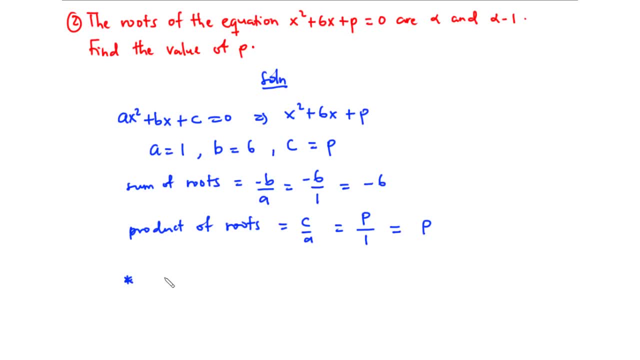 the sum of roots and the product of roots. so for sum of roots that is alpha plus alpha, minus 1. so alpha plus alpha is 2 alpha and then minus 1. so let's call this equation 3, this equation 1 and then this equation 2. 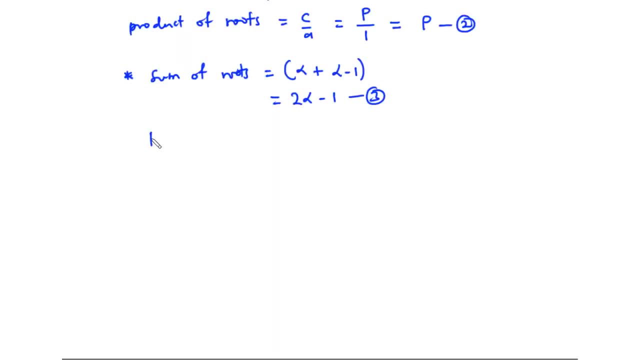 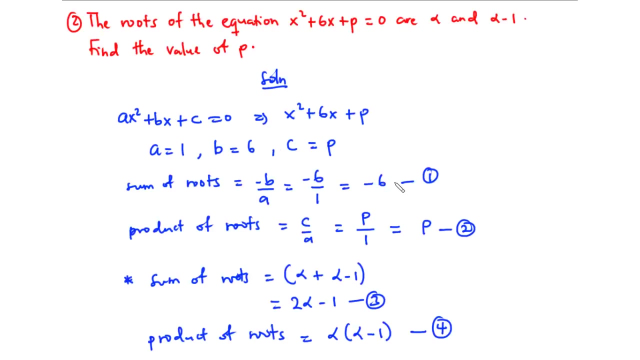 now to the product of roots. so we are going to multiply alpha and then alpha minus 1, so this is the expression for the product of roots. let's call this equation 4, so here we have sum of roots equals negative 6, and then sum of roots equals 2 alpha minus 1. 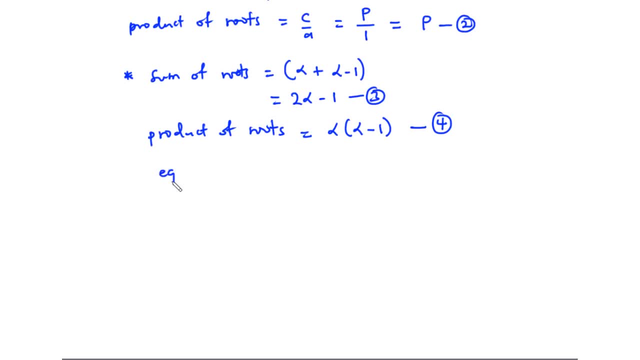 so we say equation 2: 1 is equal to equation 3. so we have the sum of roots to be negative 6, yes, negative 6, and that is equal to equation 3: 2 alpha minus 1. now let's transpose negative 1 to the left hand side. 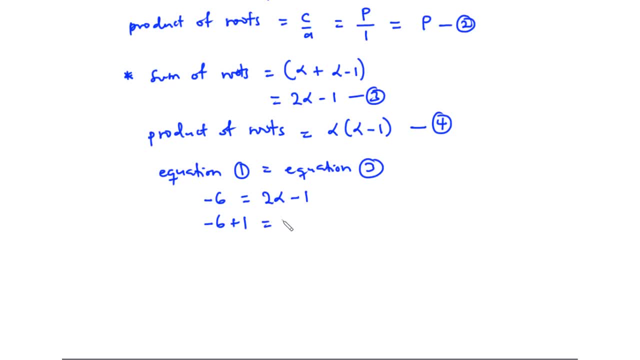 so we have: negative 6 plus 1 equals 2 alpha. negative 6 plus 1 is negative 5. that is equal to 2 alpha we divide through by 2 and then we have alpha to be negative 5 over 2. so this is alpha. 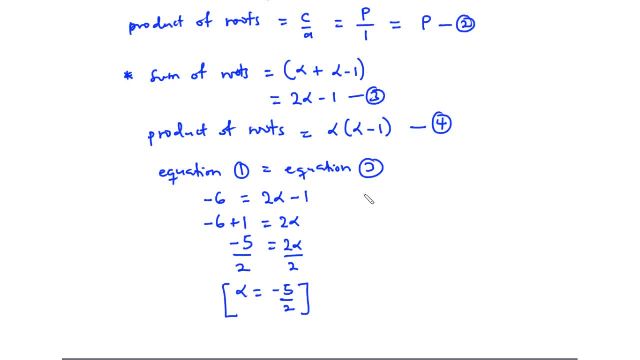 now, since we are interested in the value of p, we are going to equate equation 2 to equation 4. so we say equation 2 is equal to equation 4. so we have p equals alpha times alpha minus 1. so from here we have alpha to be negative 5 over 2.